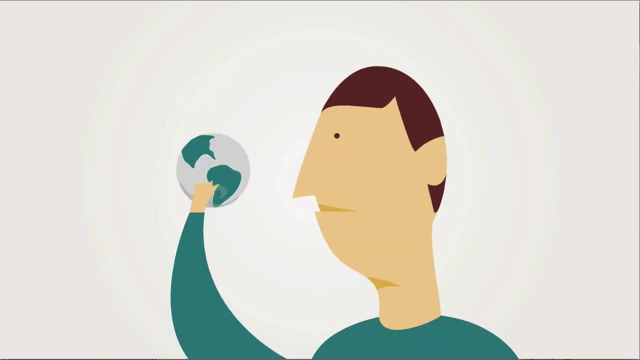 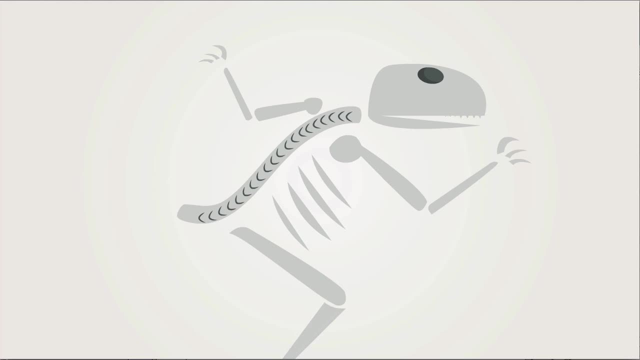 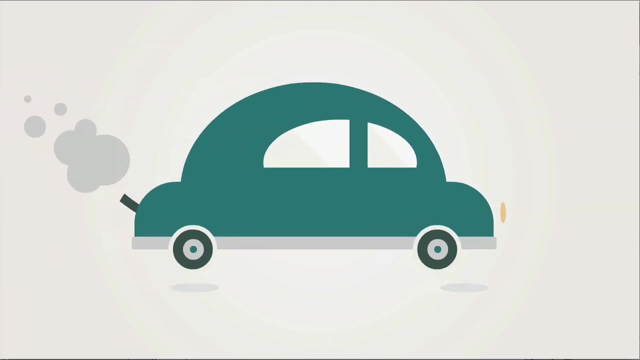 change. To understand human-induced climate change or global warming, we need to understand something about burning fossil fuels. Fossil fuels are the remains of living things from millions of years ago, mainly composed of carbon with varying amounts of hydrogen. If you collect all the exhaust gases from your car during a journey and squash them into, 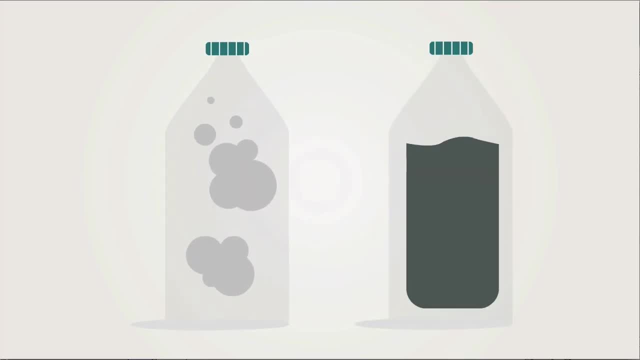 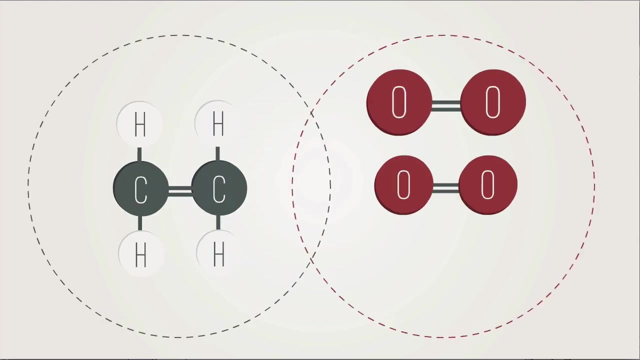 a bottle so that they can be weighed compared with the weight of petrol burnt. the exhaust gases will weigh much heavier than the petrol because oxygen from the air has been added. Here is a bit of a petrol molecule: H2CCH2.. When the fuel burns it joins with six oxygen. 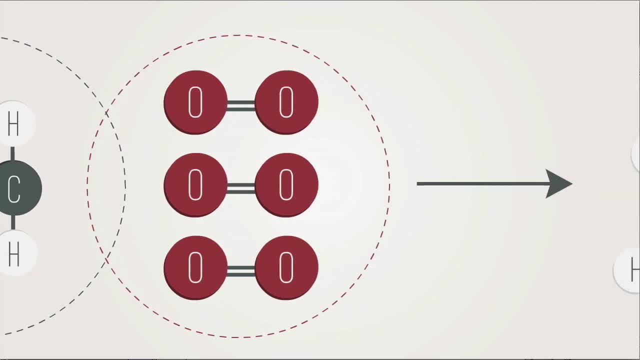 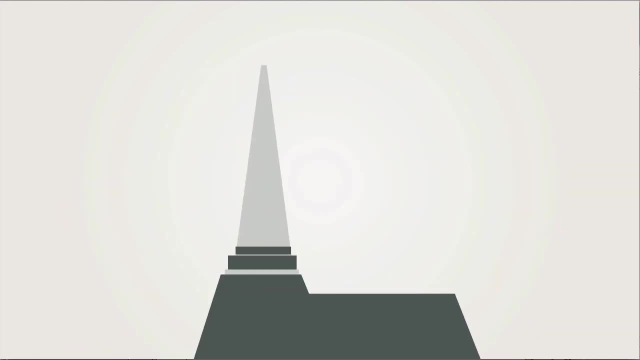 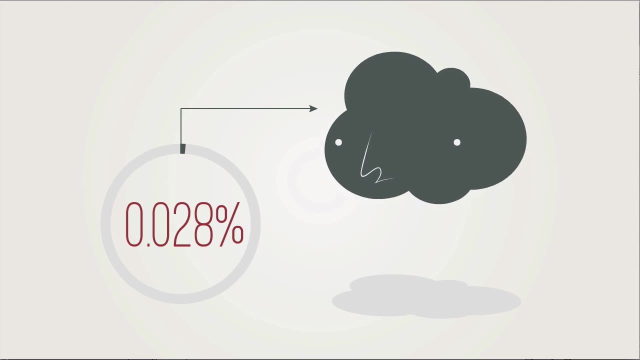 atoms or three molecules to build up hydrogen oxide or water vapour. that's two molecules, and carbon dioxide, another two molecules. Before the world became industrialised by burning fossil fuels, the carbon dioxide concentration in the atmosphere was about 0.28%- tiny compared. 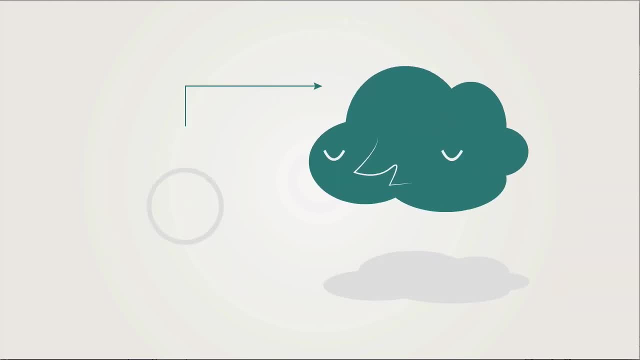 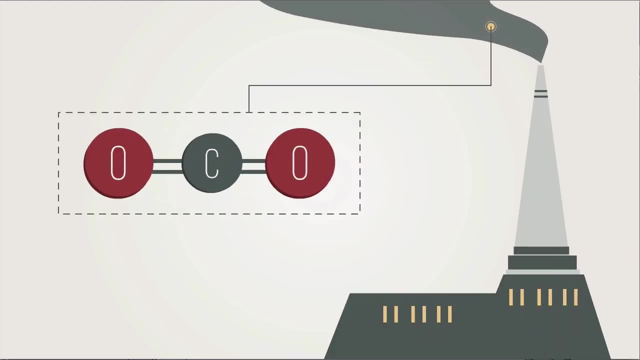 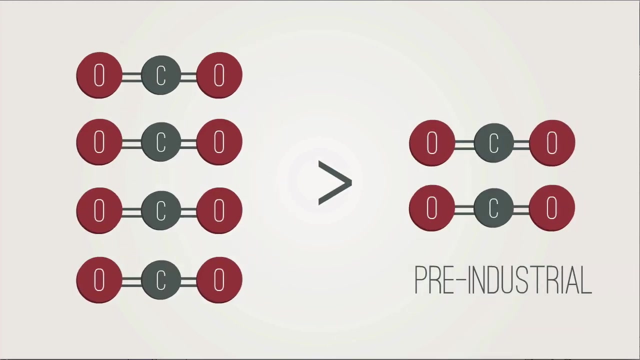 with oxygen at 21% and nitrogen at 78%, but enough to keep us warm. But this carbon dioxide released when fossil fuels burn adds to the existing carbon dioxide levels, which are now nearly 50% higher than in pre-industrial times, Although we get a daily supply of heat. 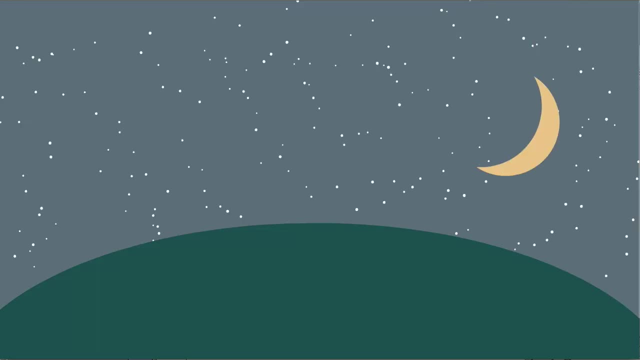 from the sun, the Earth's carbon dioxide levels are still very high. The Earth's carbon dioxide is Behagnian and because of the heat from the air it is high, and the Earth normally loses this at night and in the cooler seasons, so that the average temperature of 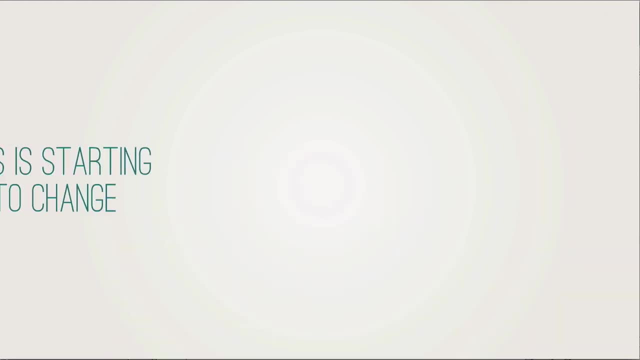 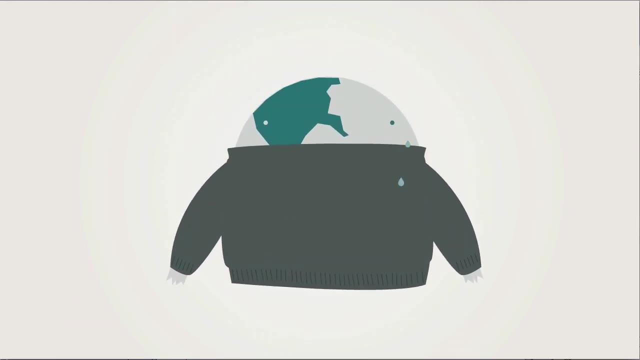 the Earth remains constant, But this status quo is starting to change As humanity adds carbon dioxide into our atmosphere. it is as if we are putting a sweater round the planet. The extra layer isolates the heat and it cannot escape as easily Whilst it. 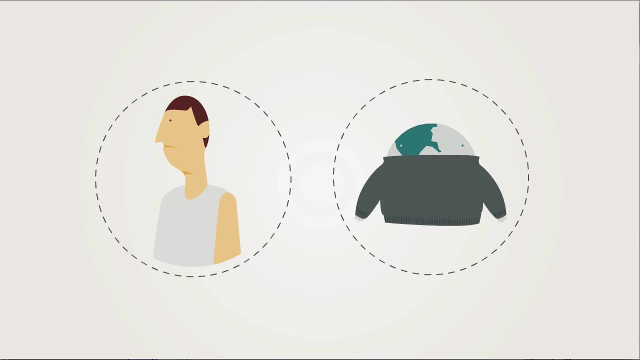 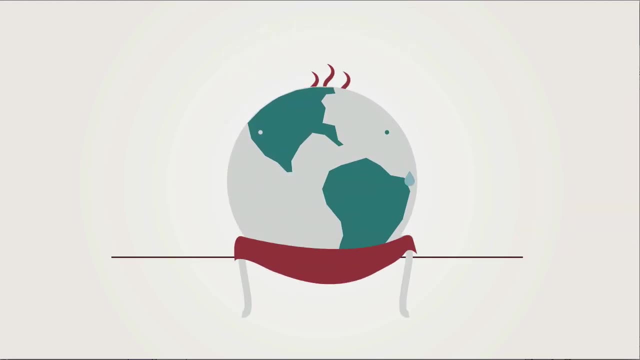 is easy to take off your sweater. the Earth cannot lose its greenhouse gases as quickly and we keep adding it back and by doing so, it will continue to do so, And there is no adding to them. By putting our planet in a sweatbox, we are causing wide-ranging consequences. 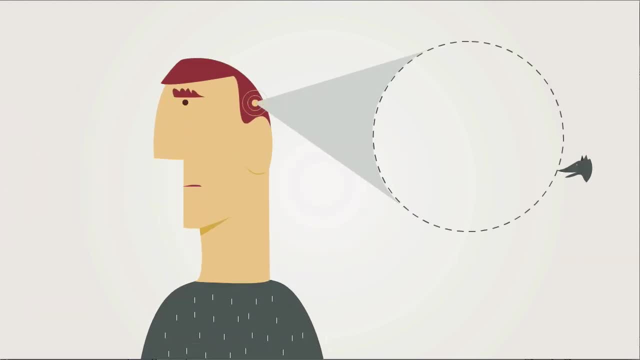 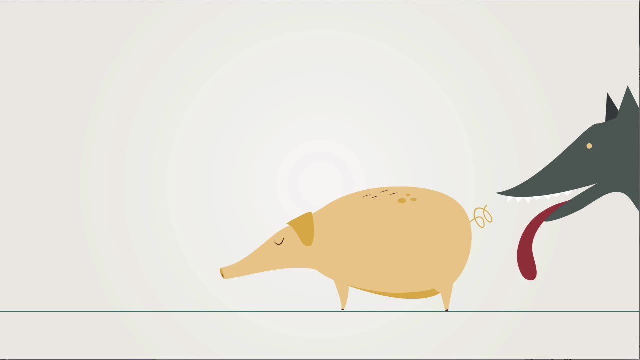 for our climate. Some people think that living things contribute to the enhanced greenhouse effect because they breathe out carbon dioxide, But this carbon has come from their food, and that's come from plants, which took carbon from the atmosphere in what is called the. 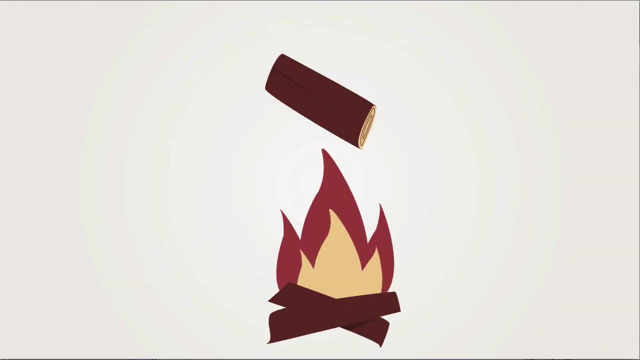 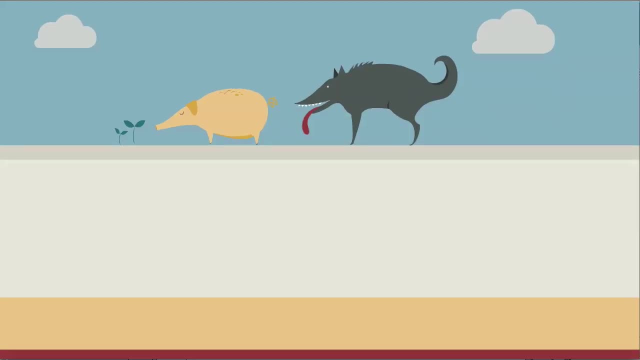 carbon cycle, and you can see the linked video for that. Even burning wood doesn't contribute to the enhanced greenhouse effect, as long as the trees you cut down are replanted. However, the carbon in fossil fuels has remained trapped underground for hundreds of millions.